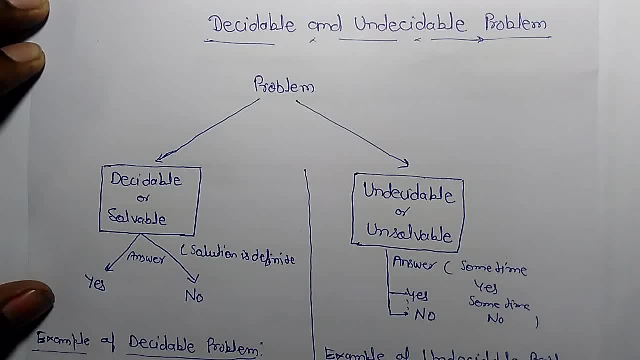 which are not solvable. And if there is an algorithm or for a particular problem and you find a solution in yes or no, then that problem is decidable. And if you find the solution in sometime yes and sometime no, then that problem is undecidable. For example, does 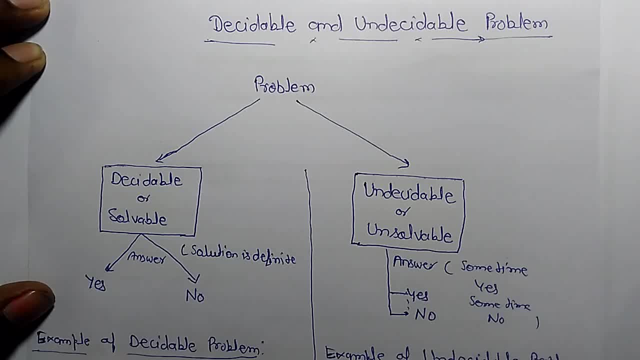 the sun rises in the east. Answer is yes. Does the sun rise in the east? Yes, This is the decidable problem. Does the earth move around the sun? Yes, Answer is yes, So it is also a decidable problem. Sometime we see that if some person is working in private. 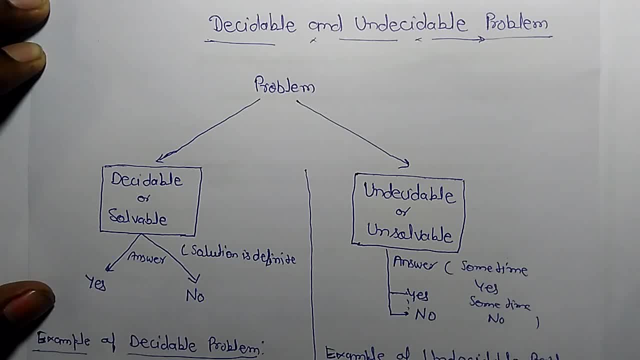 or government And I ask that person: are you a private employee? That person can give answer in yes or no. So that is a decidable problem In undecidable problem. if I ask someone: will tomorrow be a rainy day? So it is not decidable Where tomorrow would be a rainy day or not. It is. 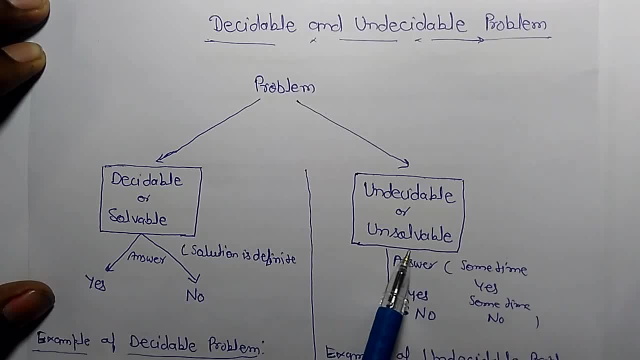 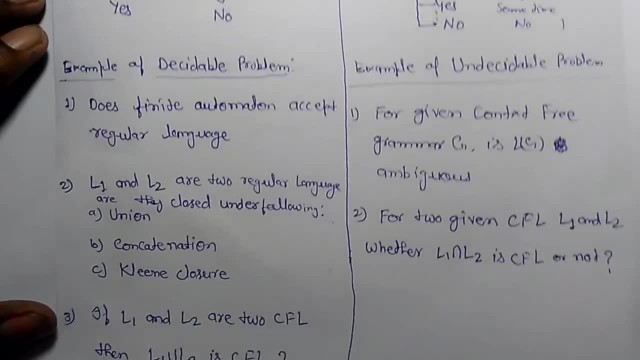 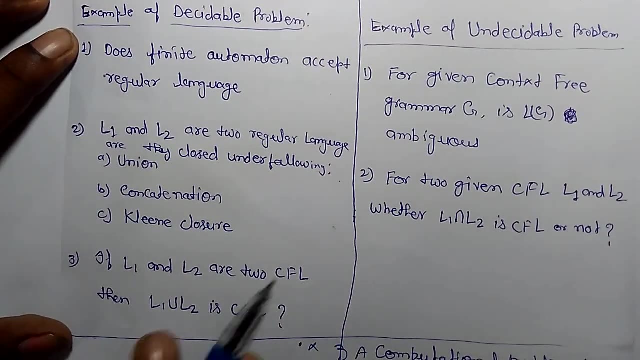 completely depend on nature, So it is undecidable. It may be a rainy day or it may not be a rainy day. In TOC the decidable and undecidable problems. examples are: Does finite automata accept regular languages? Yes, we can decide it. check that particular language is correct. will it accept finite automata? 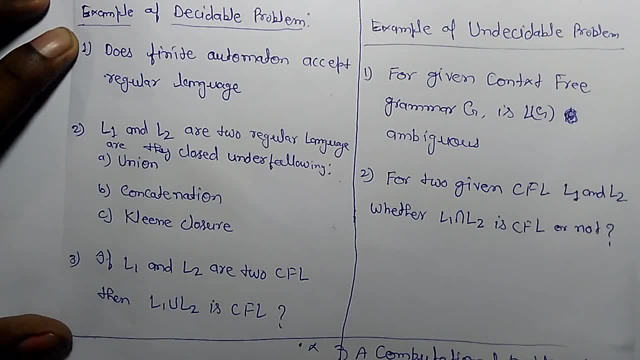 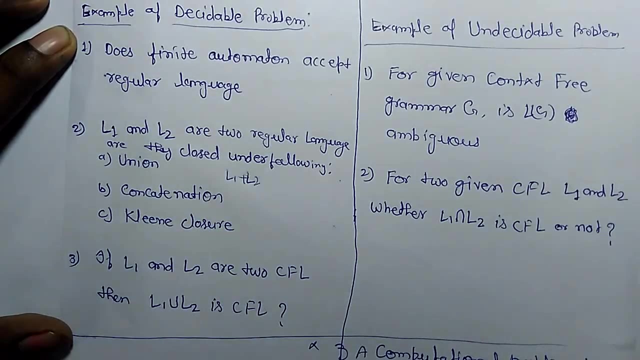 or not? Answer: percentage of data registered. If learning is pattern generated, Terrestrial input is L2. are two regular languages? are they closed under following condition: union L1 plus L2. can we decide it where this would be a regular language or not? yes, we can decide it similarly.